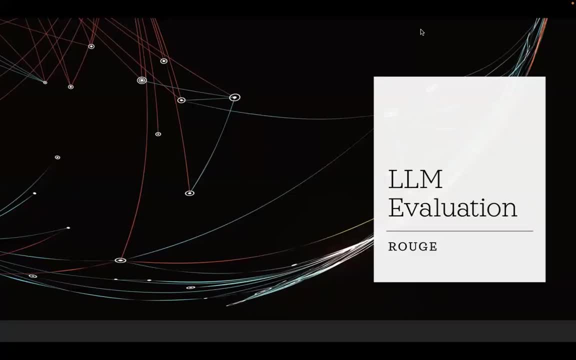 classification models and all the outputs are deterministic. The prediction, the ground, truth are deterministic. In case of language models, when we ask a question and get an answer, or when we ask the language model to summarize, the output is non-deterministic And it varies from one experiment to the other. 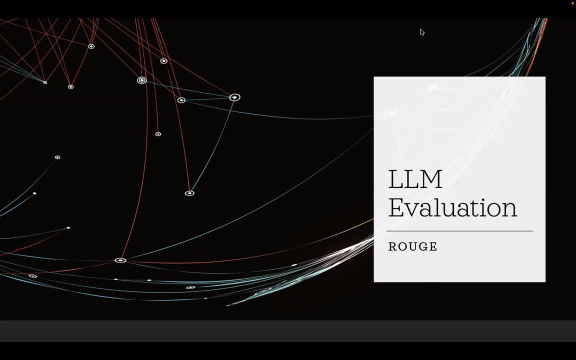 So we have to see whether we can get the exact same result. We have to see if we can get the same result or if we can get the same result. So in this case we can get the same result. So the language model is actually a challenge in how we evaluate the quality of the output. 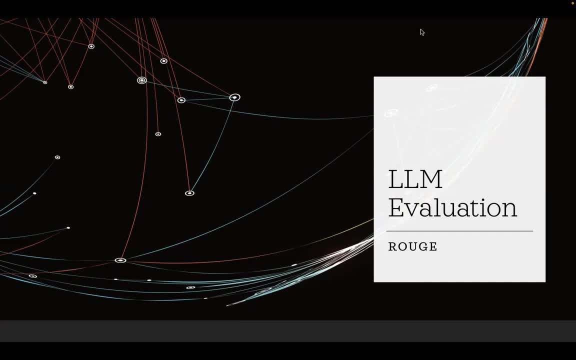 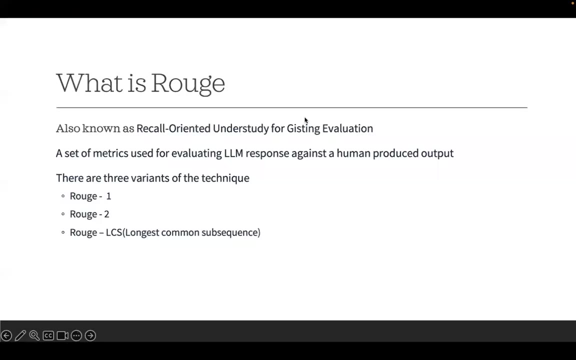 from language models. So a rouge matrix is one of the techniques by which we can evaluate the responses from the language models. So let's see what it is. So after we look at the theoretical part of the rouge matrix, I will show a slide of a. 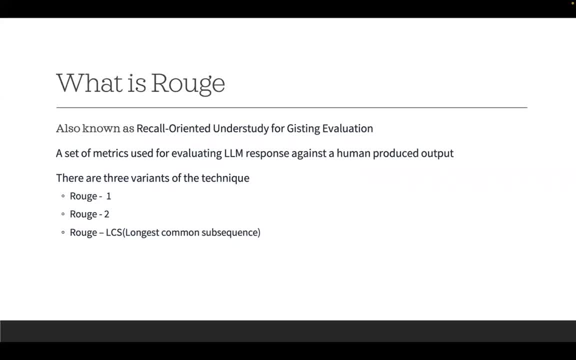 Python implementation of that also. In fact, in my GitHub I have put a repo on prompt evaluators and I plan to add more techniques. Rouge is just one of the techniques. Now Rouge is also known as a recall-oriented understudy of gisting evaluation. 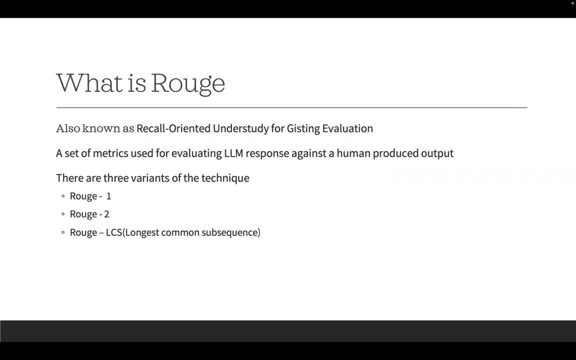 It is a set of metrics used for evaluating LLM response against a human-produced output. So if I have a golden set of question and answer, I can then use that golden set, which is the human-produced output, compare it against the language model response and then generate some metrics. 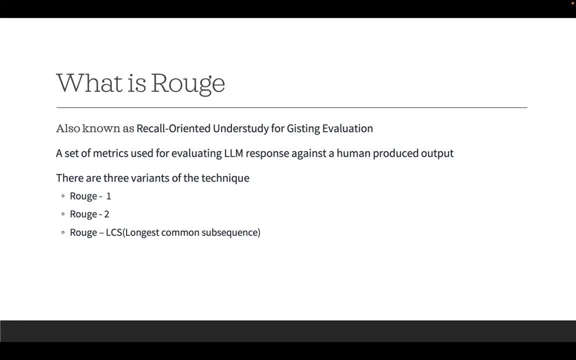 Now there are three variants of the Rouge technique, or three variants of how we calculate the metrics. The first one is called Rouge 1, which is based on unigrams of the response, and we'll see soon what it is. Rouge 2 is bigram and Rouge LCS is the longest common subsequence. 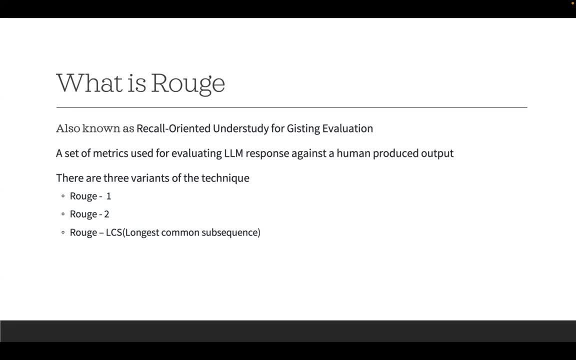 We identify the longest common subsequence between the golden answer and the LLM response and then try to evaluate the response. So let's take a look at Rouge 1, first right. So let's say in our, in this example: 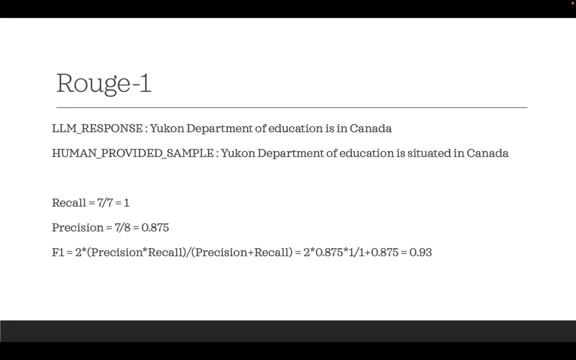 when we ask a question to LLM saying where is UConn Department of Education? Let's say the LLM response is UConn Department of Education is in Canada And the human-provided sample or the golden answer for that question is: UConn Department of Education is situated in Canada. 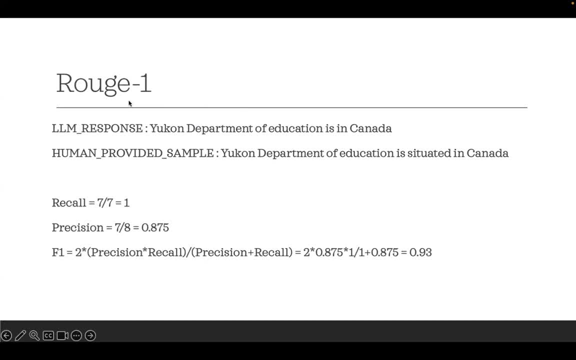 Now, in this case, in case of Rouge 1, the way we calculate the recall precision, we calculate in F1, it's like this: right. So 1 means unigram, right. So in the sentence we see how many unigrams we have. 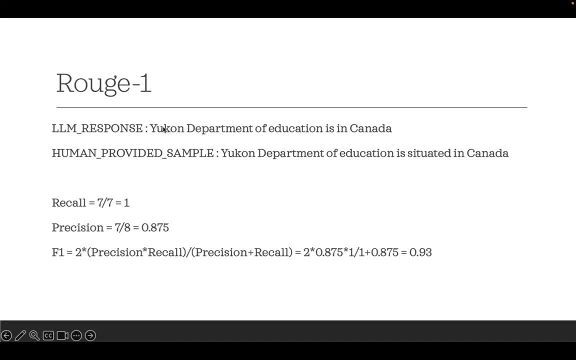 So unigram. so this is 1 unigram UConn. this is 2nd, 3rd, 4th, 5th, 6th, 7th, right. We have 7 unigrams in the LLM response. 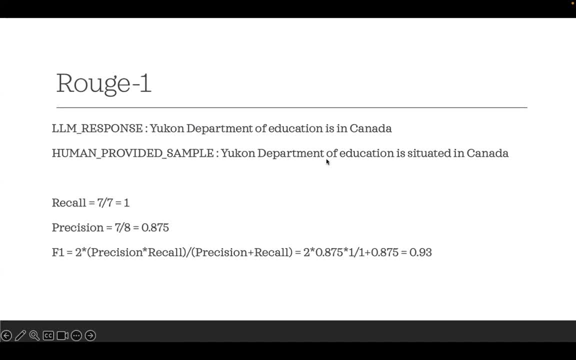 In the human-provided sample we have 1,, 2,, 3,, 4,, 5,, 6,, 7, 8.. 1,, 2,, 3,, 4,, 5,, 6,, 7, 8.. 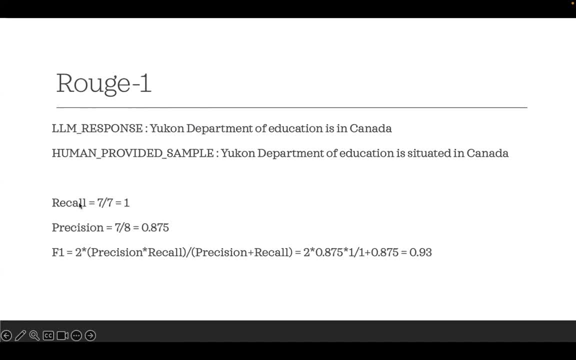 6,, 7,, 8.. Now the recall is calculated by identifying how many of these unigrams we are able to recall correctly. So, for example, unicorn is here, Unicorn is there in my LLM response, as also in my golden response. Department is also there, right. So 1,, 2,, 3,, 4,, 5, and. 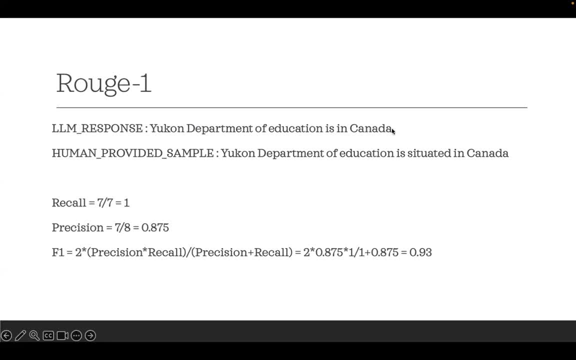 5,, 6, and 7, right. So I am able to get all the 7 unigrams recalled based on the human provided sample, right. So the recall would be then 7.. Which is the number of unigrams that I recall divided by the total number of unigrams that. 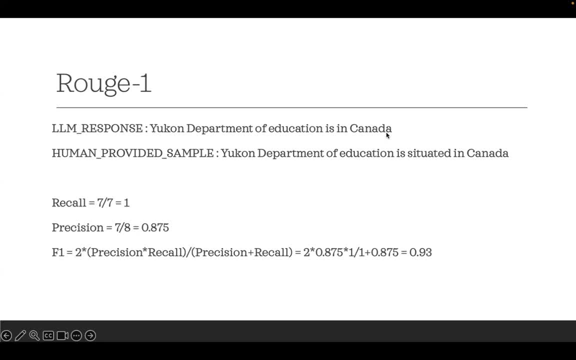 I have in my LLM response Same concept, the recall formula, same concept that we have in the traditional MLOps also, right? So we are trying to find out how many we are recalling. So it is 1 because all the 7s we are able to recall, The precision I calculate. 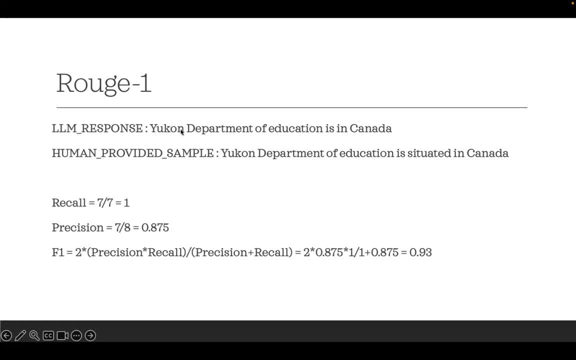 by how many of these unigrams I was able to, or the LLM response was able to predict In its response, divided by how many unigrams we have in the golden answer. In the golden answer we have 1, 2, 3, 4, 5, 6, 7, 8.. So the precision is 7 divided by 8, 0.875.. F1. 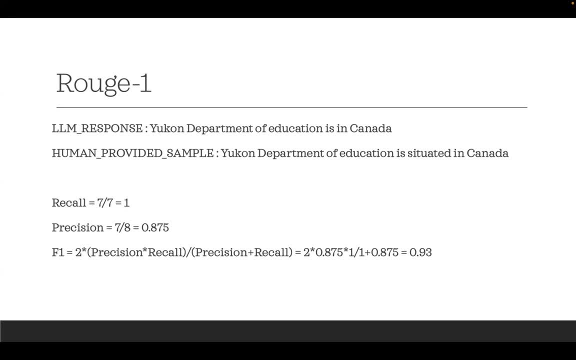 score. the calculation is 2 multiplied by precision into recall precision plus recall right, This gives me 0.93.. Now some challenges with the Rouge-1.. Is it actually does not take care of ordering of the words, right? So if I change the orders, 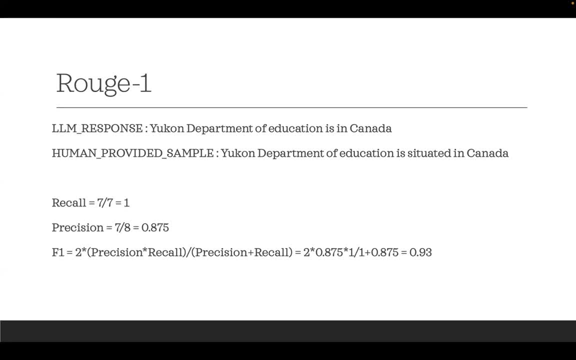 and make it like a gibberish or a haphazard sequence of words, I'll still get this score Also if I put a negative thing right. Say, UConn Department of Education is not in Canada, right In that case? also? 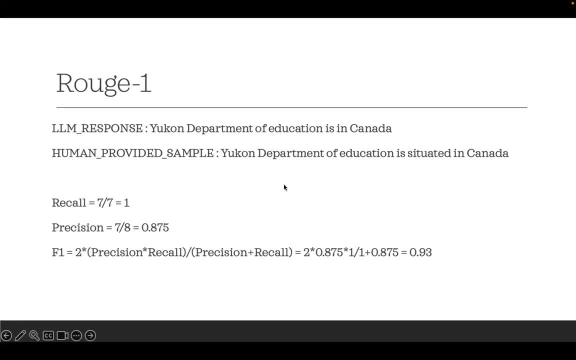 This will not be a perfect score, right? So to solve this problem somewhat, there is the Rouge-2,, which is similar technique, but instead of taking one gram now we are taking bigrams of words, right. So the same response. 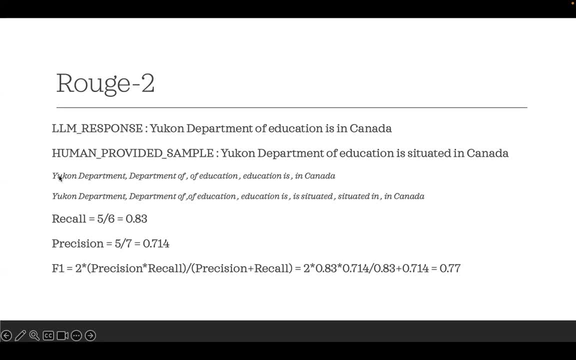 if I divide it into bigrams. so UConn Department, UConn Department. So in the LLM response we have one bigram, UConn Department, Department of is a second bigram of Education is third, Education is fourth and in Canada is fifth. So I am able to recall this: five bigrams. 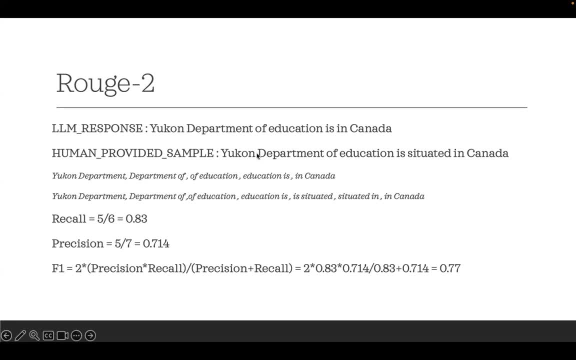 I will be able to find these bigrams in the human-provided sample as well. right UConn Department Department of Education is in Canada, So in this case the recall would be five, one, two, three, four, five divided by six, which is the total number of bigrams. 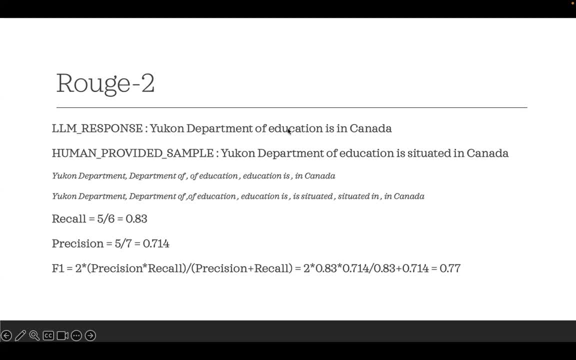 in the LLM response: One, two, three, four, five, six, five by six Precision would be again five divided by total number of bigrams in the human-provided sample: One, two, three, four, four, seven, eight and nine, And the total number of bigrams is seven total 그. 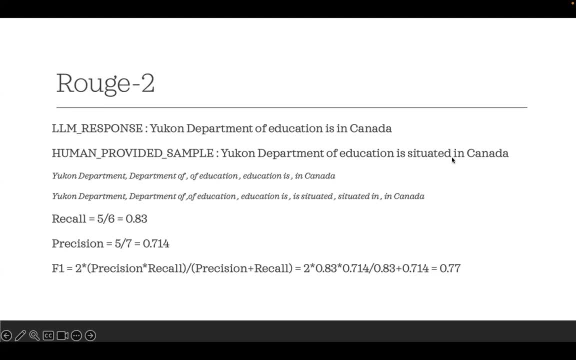 in the human-provided sample, One, two, three, four, five by sixres, menor of 6, 5, 6, 6 and 7, right 5 by 7, 0.714.. F1 equal to 2 multiplied by precision recall. 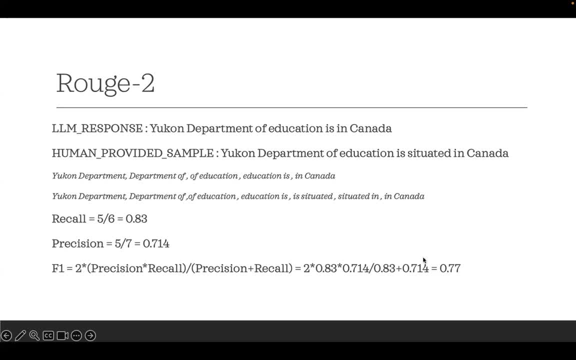 precision plus recall right Now. if you see, compared to ROUGE1, the ROUGE2 scores are relatively lower. right, We can actually, to get more, better results, we can go to trigrams, 4 grams and 5 grams also. We will not go there. But the third technique is called. 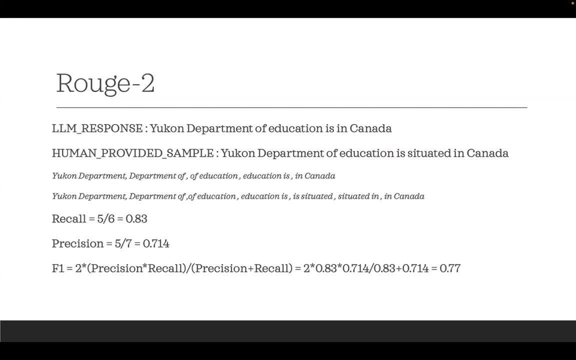 the third technique that we is the longest common subsequence, right? So what is the longest common subsequence? The longest common subsequence is where we compare the LLM response and the human provided sample and find out how many subsequence are there in these two sentences. For example, if the LLM response is this: 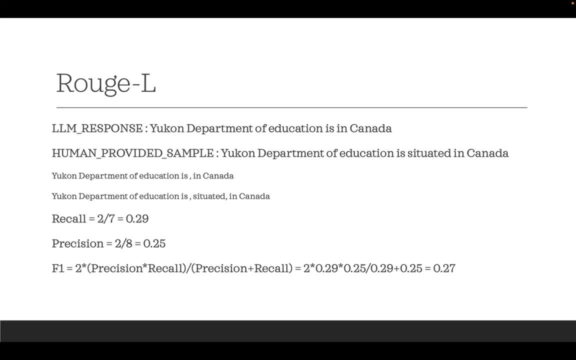 the common subsequence is UConn Department of Education is because here also I have UConn Department of Education is, and the second subsequence is UConn Department of Education is in Canada. So without a break, there are two subsequence in that. and then we calculate. 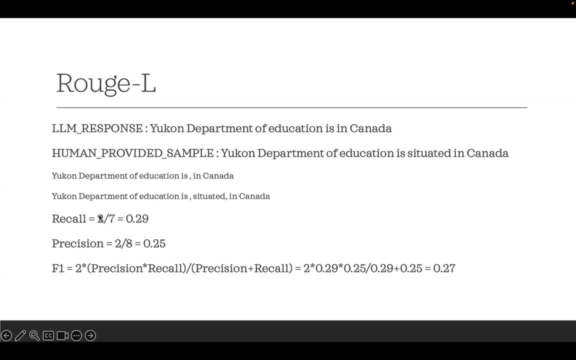 the recall precision in F1 based on that right. So I have two subsequences, but in total the denominator is the unigrams. So how many subsequence divided by total unigrams: 1,, 2,, 3,? 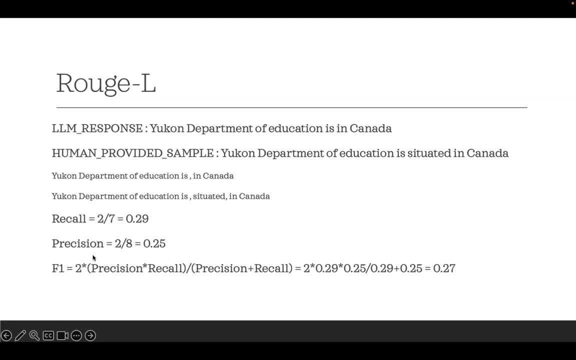 4,, 5,, 6,, 7,, 2 by 7.. Precision is again 2, which is the number of subsequence divided by total unigrams in the human provided sample: 1, 2,, 3,, 4,, 5,, 6,, 7,, 8,, 2 by 8, and we calculate the F1 score similarly right. 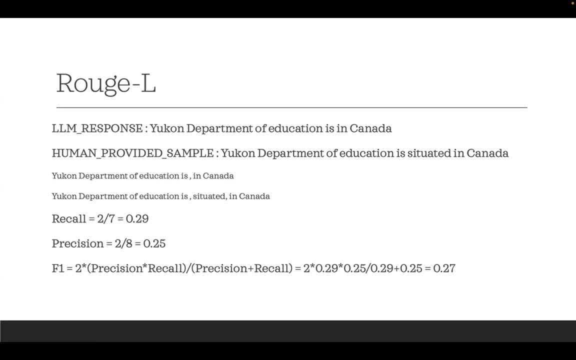 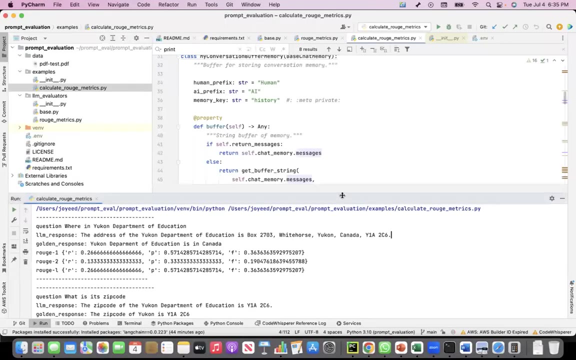 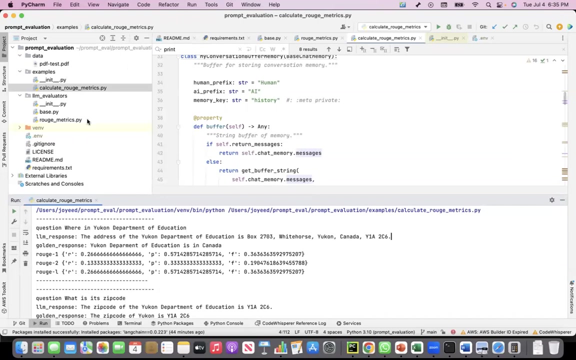 So these are the three different rouge metrics that we can use to evaluate all LLM response. Now let's see an example implementation of it using Python right, And this is something that you can find it in my repo- prompt. evolution is a repo name where I created a base class And the reason I created it as a 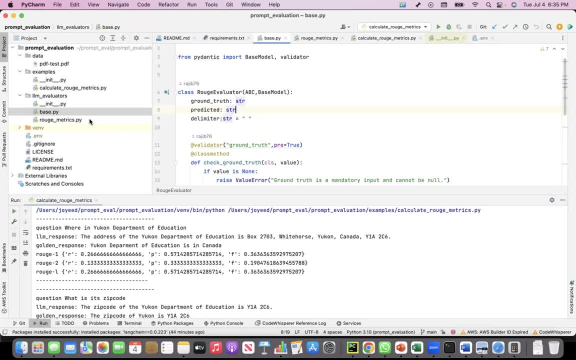 base class is. right now. I have rouge metrics. I wanted to add more metrics like the blue metrics, And then I have some idea of creating some more custom metrics, right where I can actually find out the Jaccard distance right. So 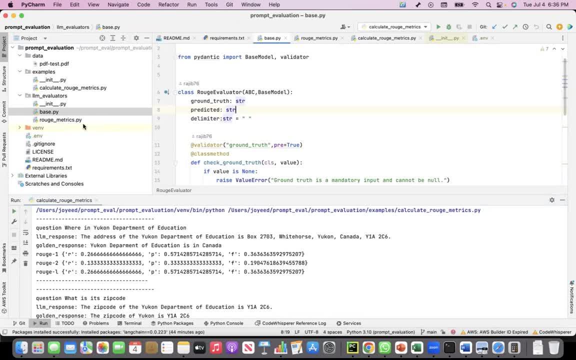 my idea is to add more metrics implementation in this repo, But for now it is how it is implemented is I have a base class right, which is the base class, is the rouge evaluator right And it, so I'm using a pidentic sum validator because I want. 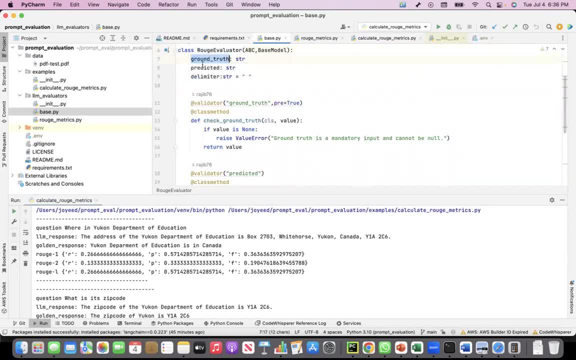 to validate that when you instantiate it, the ground truth and the predict F1 score match up those two on the predicted responses given right and there is a abstract method: evaluate. this is then implemented in the rouge matrix class where i'm using the rouge package. this is a python package. 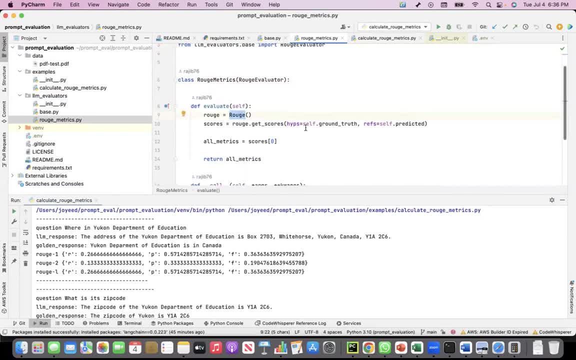 that i'm using where i'm giving the hypothesis. hypothesis is my ground truth and the reference is my golden answer. right, i'm passing this and i'm getting the scores back right. so this is, this is the package, and this is an example implementation of this evaluator. so if i go here, you'll see. 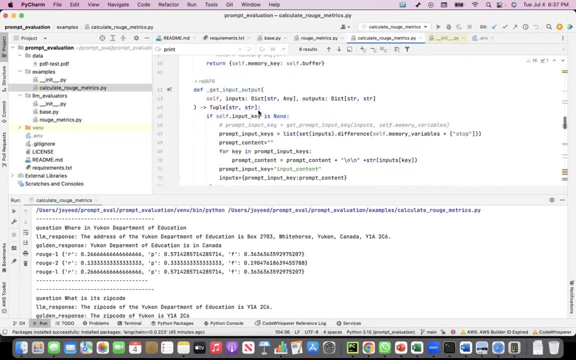 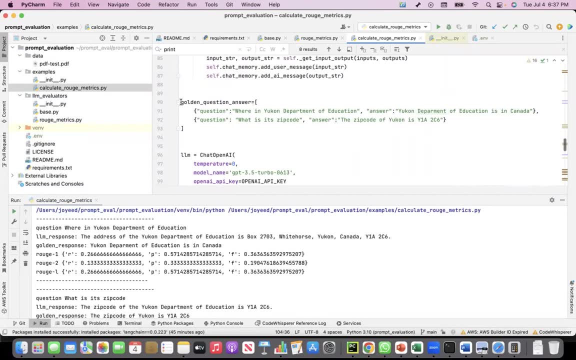 this is a normal load qa chain that i created. i will not go through the entire load qa chain. i will just show from here where i have a set of golden question and answer. the question is: where is yukon department of education? and i have the answer. what is its zip code? i have the answer. 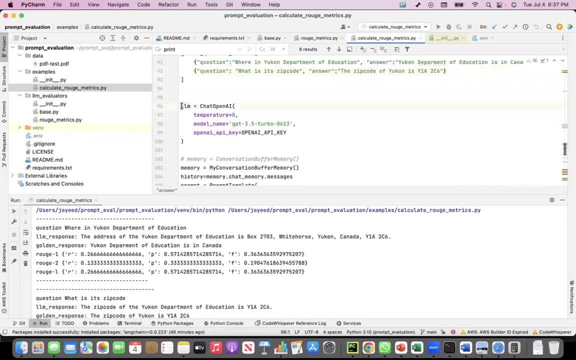 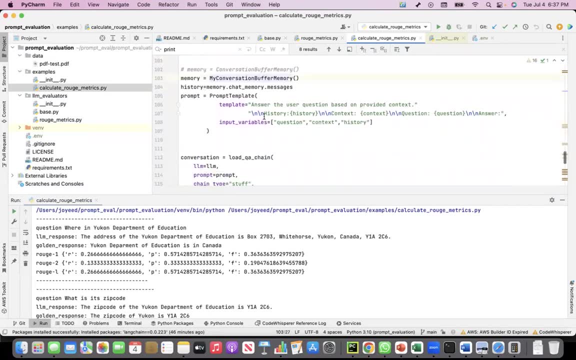 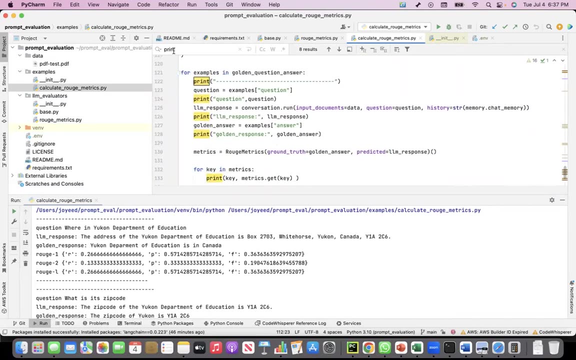 this is my golden set of question answer. i create the instance of the llm. i'm using gpt 3.5 turbo 613. i used a memory here, my prompt template. i create the load qa chain. and finally, here i am now looping over the examples that i have in my golden question answer. 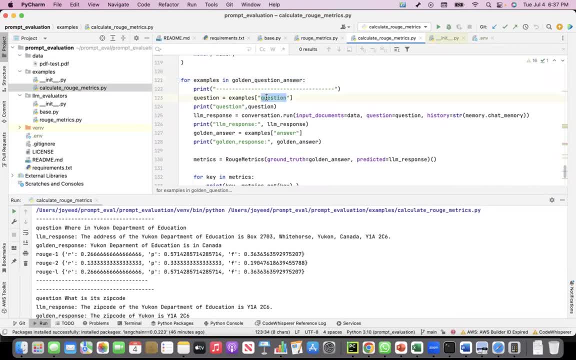 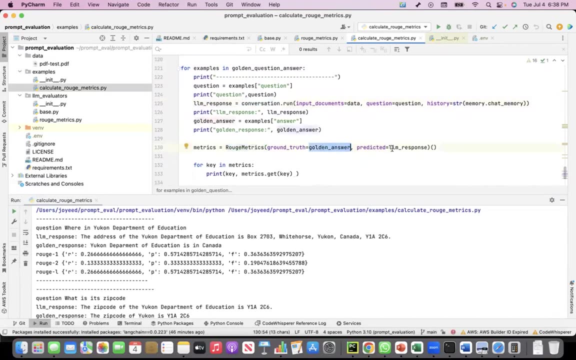 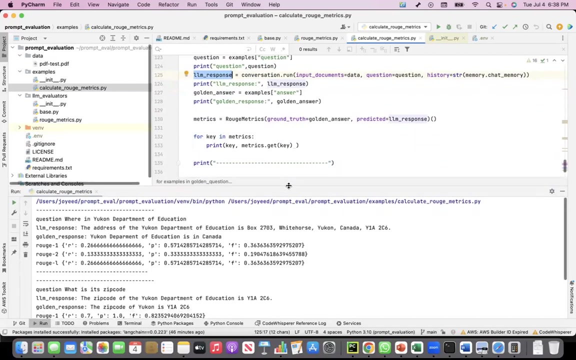 for each of them. i get the question, i get the response by from the language model right, and then i calculate the rouge matrix by passing the golden answer and the predicted is my llm response right. and i do it, for i have two examples. so that's why it is in a loop and let me run it. 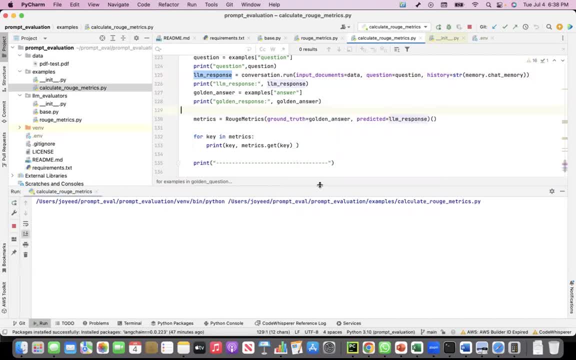 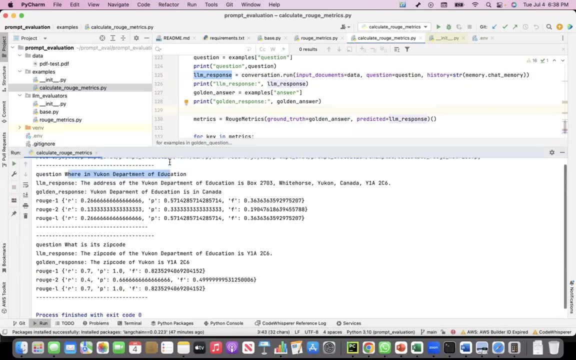 again and you will see what it so here. the question was: where is yukon department of education? llm response was: the address of the yukon department of education. Department of Education is so this is actually. I'm doing it in context learning. I have a PDF. 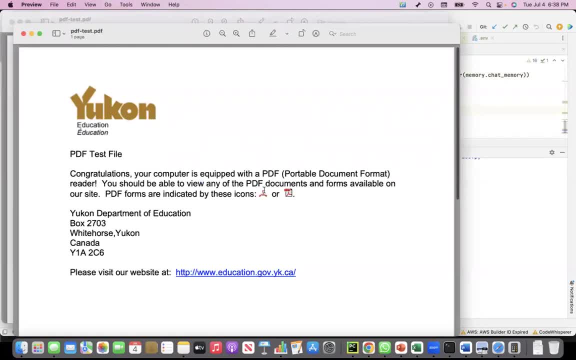 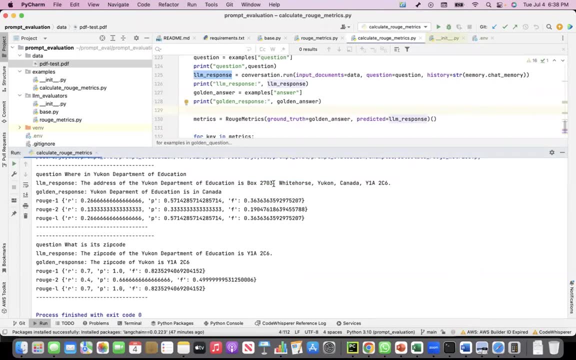 This is the PDF right where I ingested this and from there I'm doing the question and answer. right? So it is saying the address of the UConn Department of Education is box 2703, UConn, Canada. Golden response was: UConn Department of Education is in Canada, right? 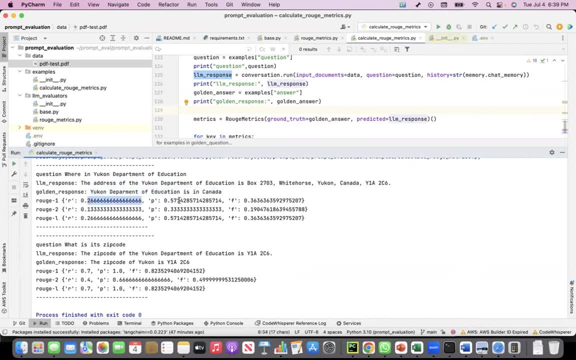 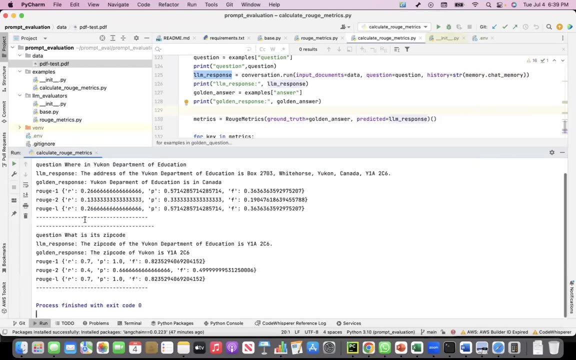 So this is Rouge 1 matrix. This is the recall value precision F1 score right Rouge 2, which is relatively lower. if you see, and this is the Rouge LCS, the longest common subsequence for the first question, and this is the zip code. What is the zip code? The LLM response. 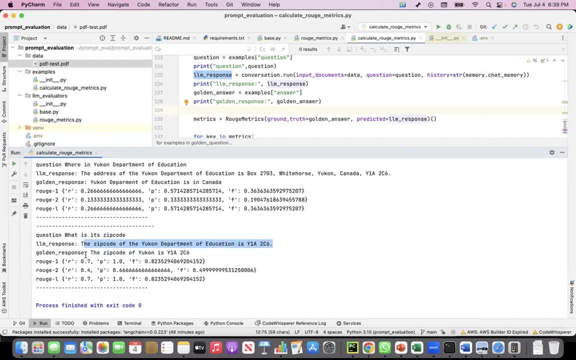 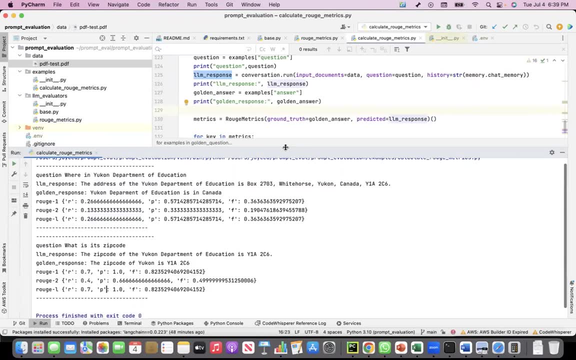 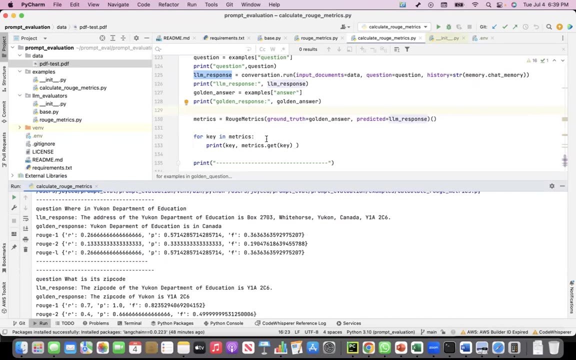 for the zip code of UConn Department of Education is this and golden response: is the zip code of UConn. is this right? And these are the Rouge matrix for that. So this is a simple implementation of the Rouge matrix. I will continue to add more metrics or LLM evaluation techniques in this. 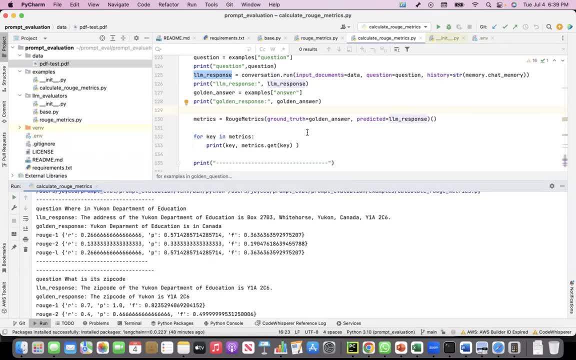 repo. Next, I'm thinking to do the blue BLEU and I have some idea on creating some custom metrics also, which may be more accurate where I can do similar discourse right. So stay tuned. Um, as soon as I. 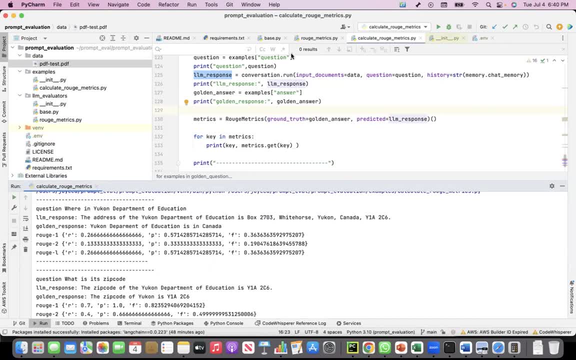 uh. add more uh metrics. I will create another recording and share it with all. Thank you, That's all.